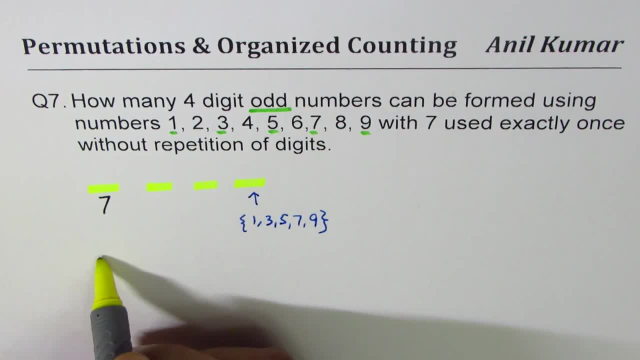 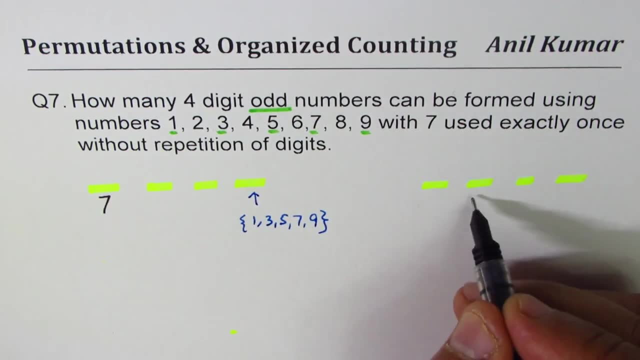 The other choice could be: let us say, let us say, let me draw it here- 1,, 2,, 3,, 4.. We can place seven in the second position, Or we could place seven in the third position. 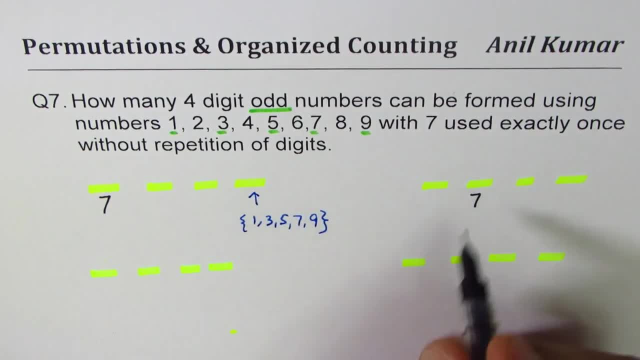 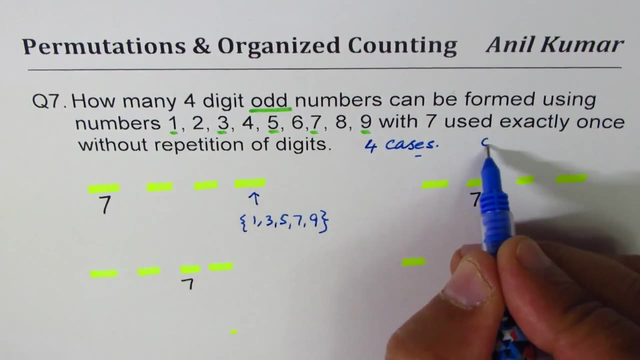 Or in the last position, Is it okay? So seven could take one of these positions, Is it okay? Only once it has been used. So these become four different cases. So we are working with cases, So four cases With odd condition, Is it okay? 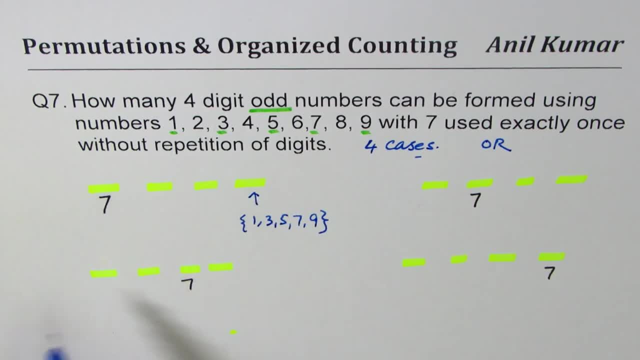 Because seven could be in thousandth place, hundredth place, tenth place or in one's place. Now let's see, If I place seven on the thousandth place, the numbers which I can fit in these three places will be what. 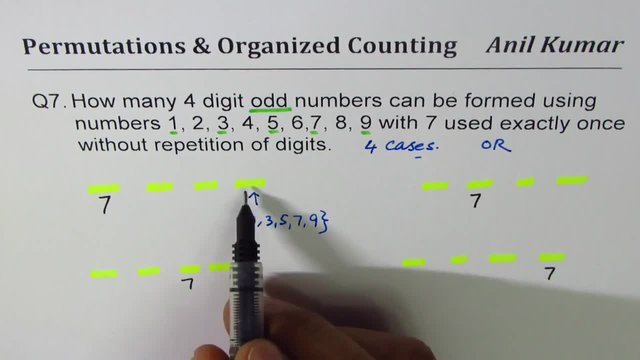 Now looking into this, it is better to fill in the last position first, Correct, Since in the last position we have some restrictions. So we have already taken away seven. We are left with numbers one, three, five and nine. 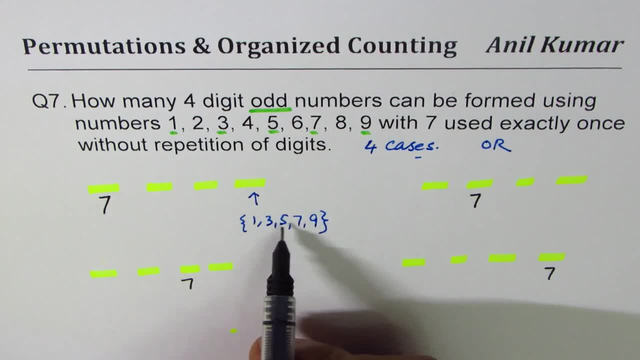 Correct, So we'll put one of those. So one, three, five and nine, So we have four choices Now, once you take away two numbers from nine, you are left with nine minus two, which is seven. We could put seven here. 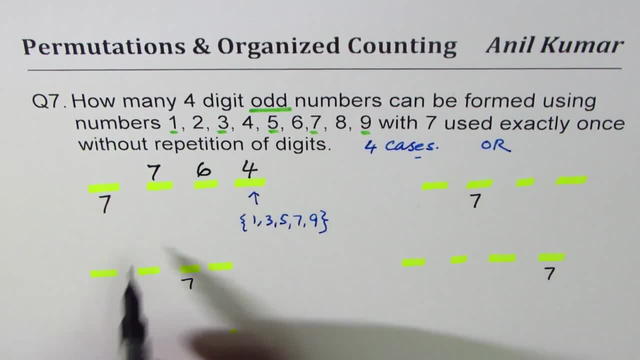 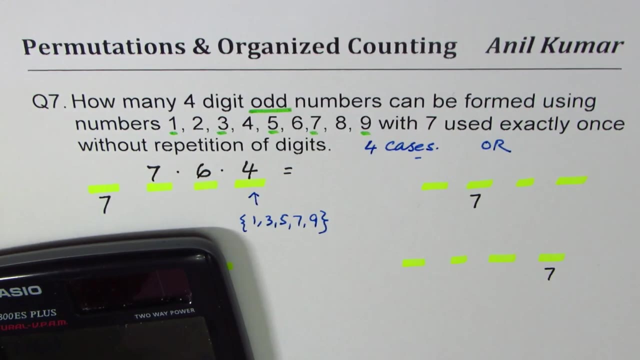 And once you place number here, we have six choices. So that becomes the combination: Multiplying seven, six and four will give us total amount of choices worth seven in thousandth place Right. So seven times six times four is equal to 168.. 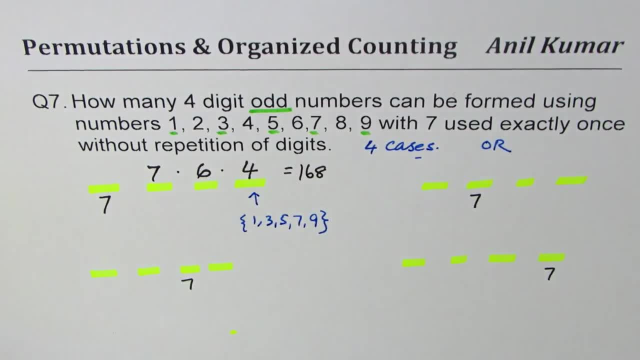 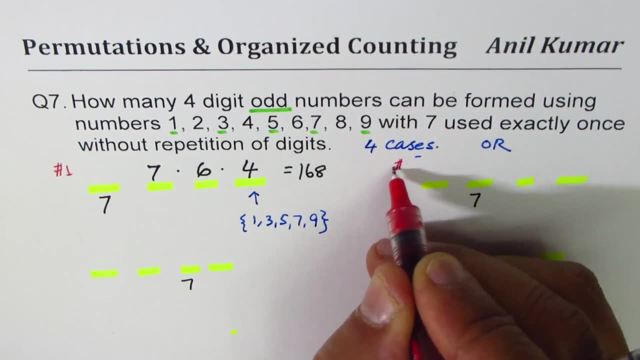 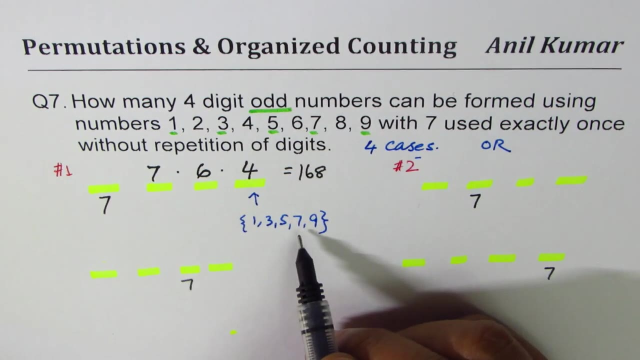 So in case one we have 168 ways. So this is our case number one. Let's see what happens in case number two. If seven is in the second position, since seven is itself odd number, we can only place four numbers in the last position. 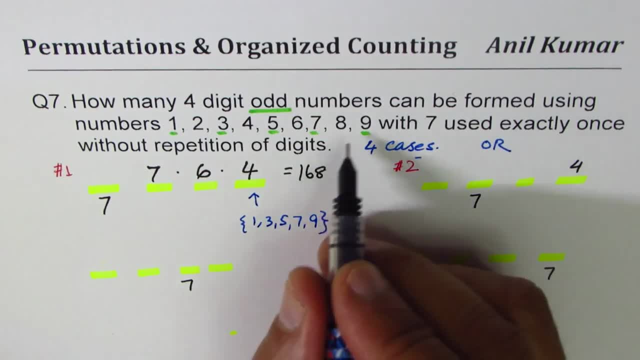 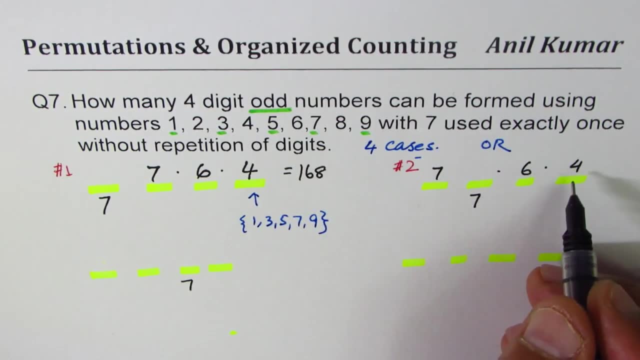 One's place. Two have been consumed out of nine. We are left with seven. Third has been consumed, Left with six. So we get exactly seven times six times four, which is again 168.. Is it okay? In this case also, seven is already taken in tenth place.